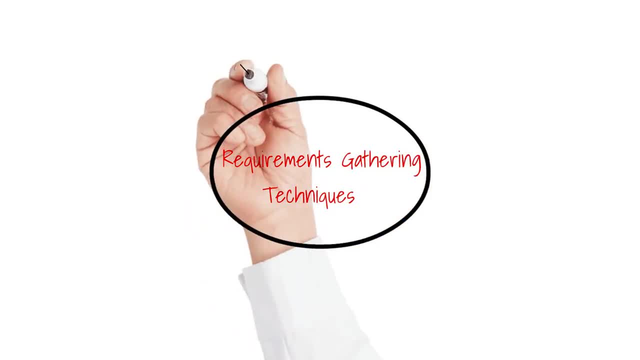 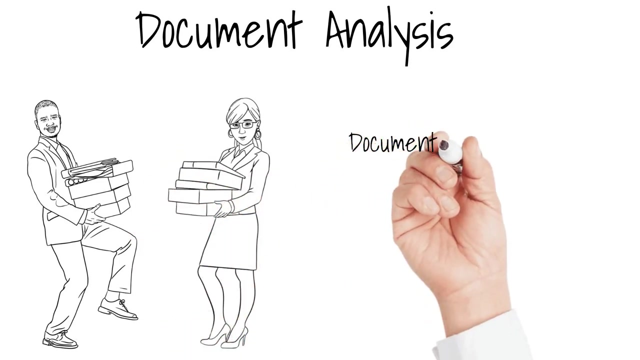 for business analysts are out there for requirements gathering. The very first technique is document-based analysis. Like the name says, it's all about documents here, not about users, stakeholders or the clients. Here the first step is to gather all the documents available and relevant for your case. 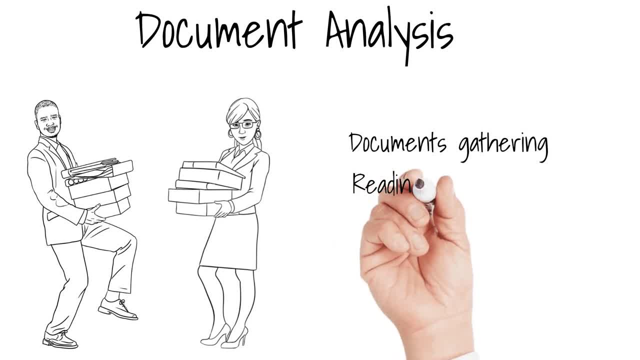 This means there is a lot of reading involved. Requirements documents can be very long, so be patient. Key is to understand the system by reading the documents, So you're able to build a baseline of knowledge which is very helpful throughout the whole requirements gathering process. 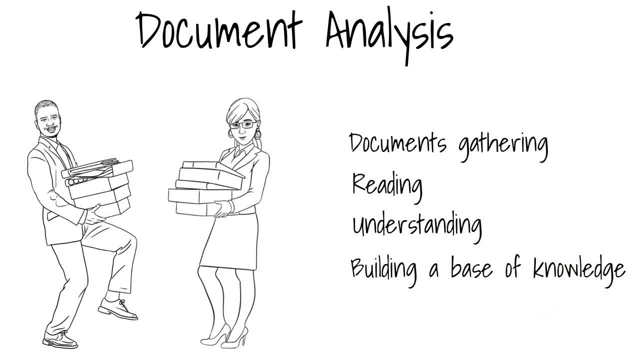 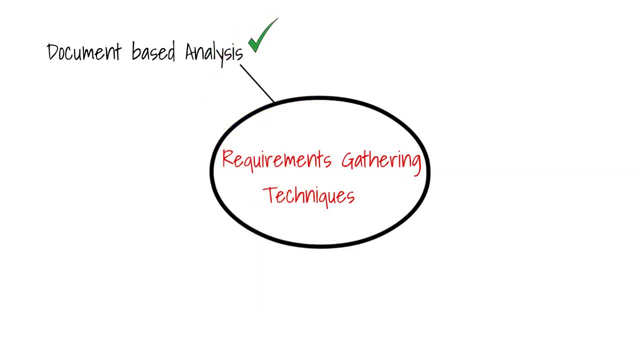 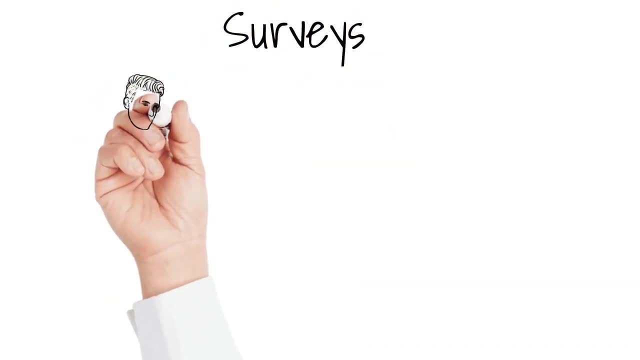 This requirements gathering technique is pretty much used every single time. It's basically the starting point in requirements analysis. The very next technique I want to cover are surveys and questionnaires. Surveys are a great tool to collect answers on standardized questions, so it's perfect for getting a high 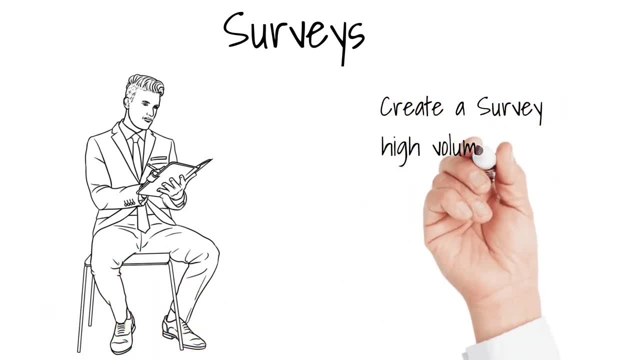 volume of data because you can easily send the survey to hundreds of people and get their insights and you don't have to talk to them one by one. You can include open and closed questions And especially for closed questions, it is easy to evaluate. 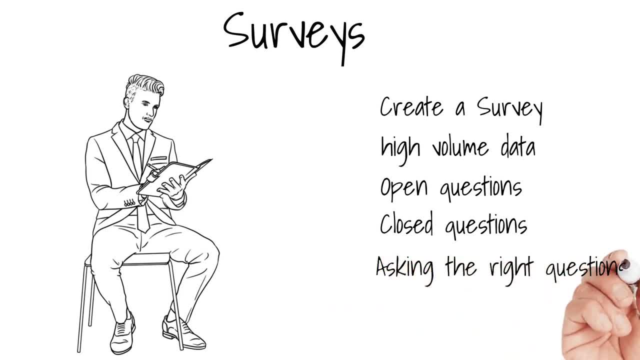 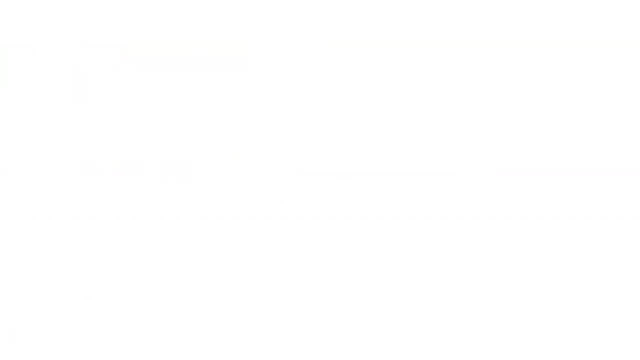 The issue here is really that asking the right questions is a challenge, And you also don't want to influence participants with the question themselves, because they could bias. Let's jump to the next requirements: gathering techniques for a business analyst- Shadowing: Shadowing is to accompany a user or a stakeholder. 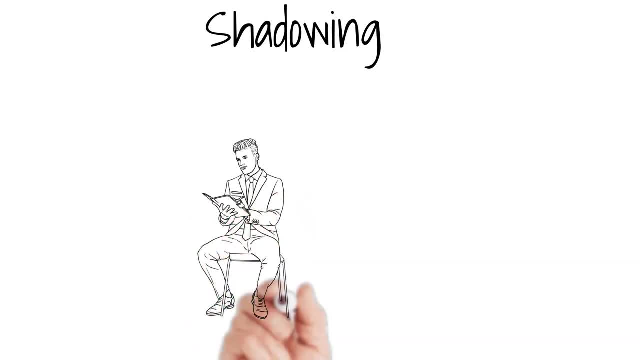 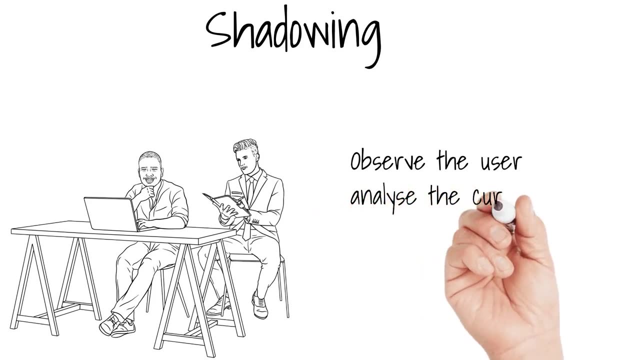 By this you're living the process the user goes through every single day. That's a powerful technique, because you're also able to perceive what I call silent requirements. Silent requirements are requirements your stakeholder won't tell you because they are so self-evident for them. 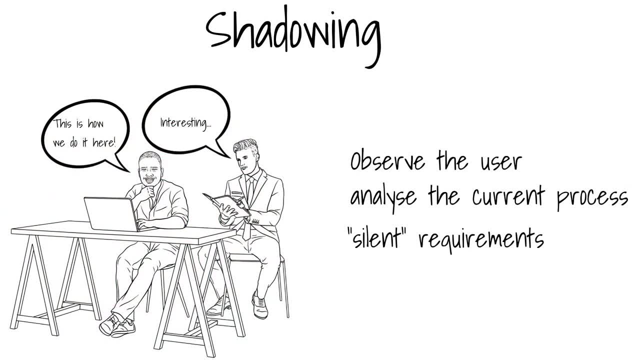 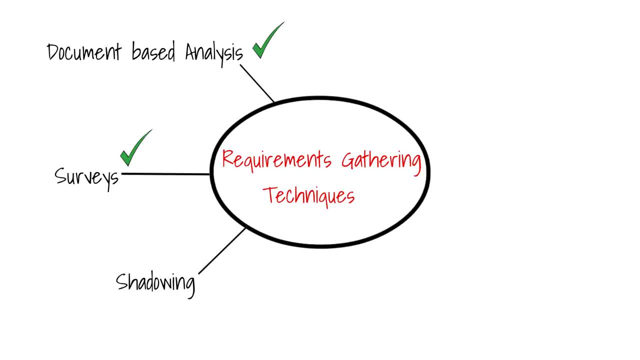 The downside here for sure is that it's very time consuming for you, as a business analyst, to shadow multiple stakeholders. Shadowing is a technique that allows you to see what's going on. Now let's go to the probably most used technique, at least for me. 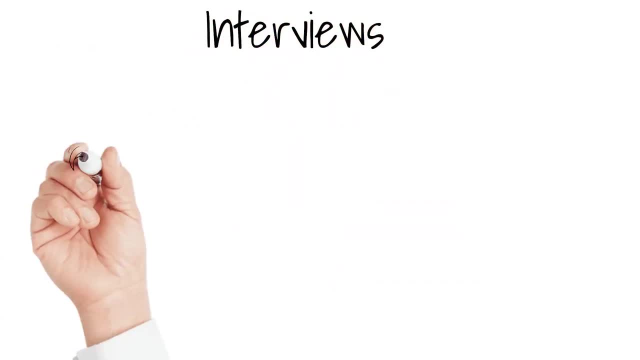 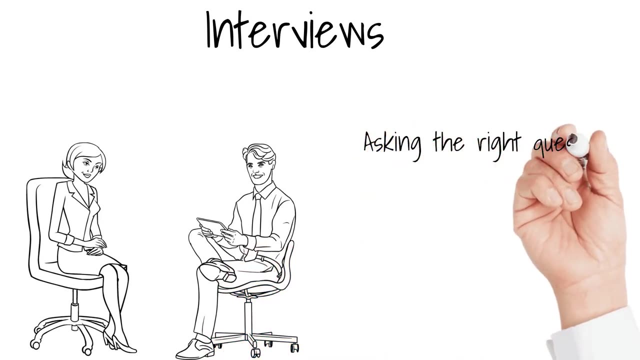 Interviews. Interviews are basically that. what service cannot provide to you For having someone in an interview, you can get very specific And also you're able to get feedback instantly. So there is a question answer loop where you can dive deeper with follow-up questions. 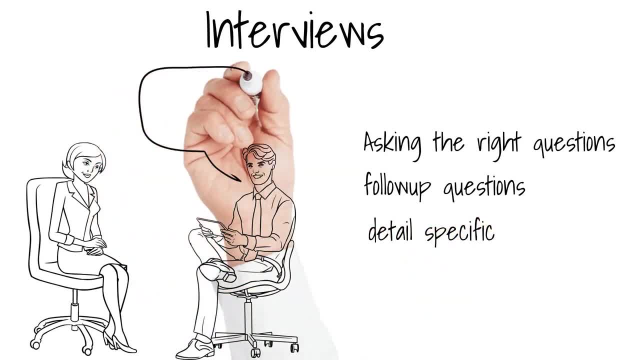 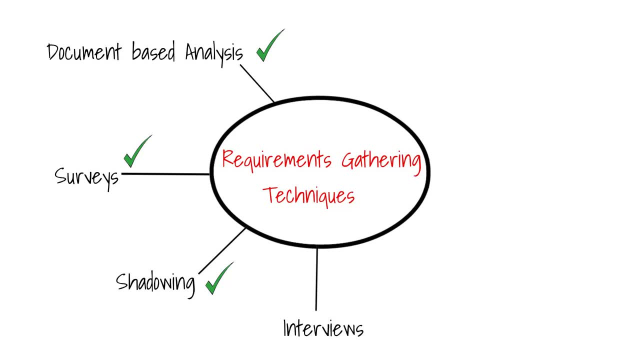 to really get down to the root. Requirements are most of the time something very specific, So it actually is pretty much necessary to dive deeper. The next requirements gathering technique I want to show you is the workshop. A workshop is not only an interview. 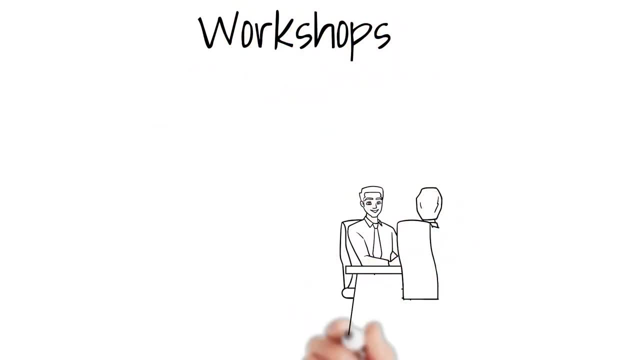 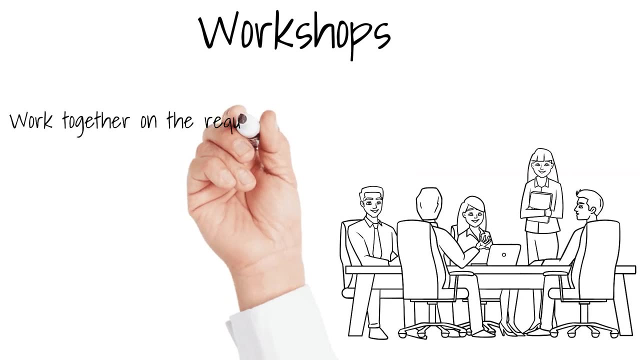 A workshop involves many people at once and also enables them to work together on specifying the requirements. A workshop is not only an interview. A workshop involves many people at once and also enables them to work together on specifying the requirements. Here the role of the business analyst. so you? 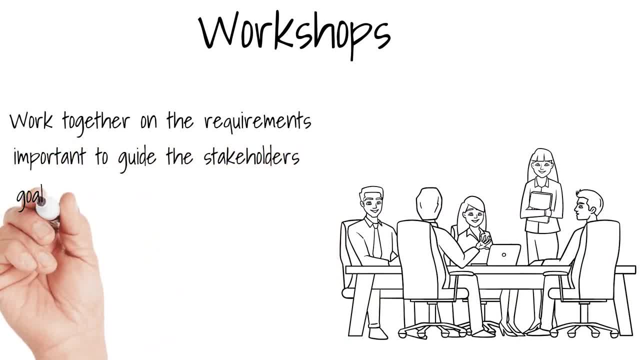 is also to ensure to guide the stakeholders at the table into the right direction, So people don't get lost. The goal definition or the desired outcome of the session is important Because when many people sit around a table for a long time, that's very costly. 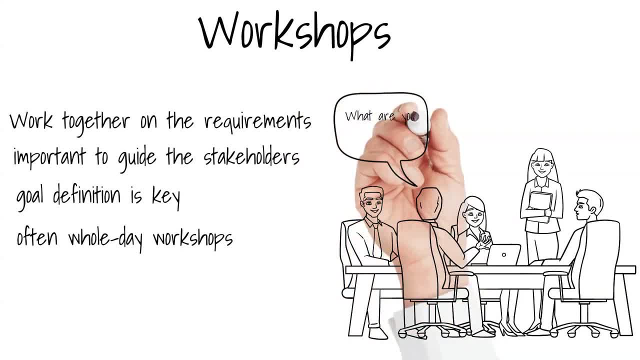 These workshops can go over hours or even full days, as per my experience, And if you have seniors also on the table, you can imagine how much such a workshop costs in the end. So better make sure to get the outcome After clarifying the workshop. 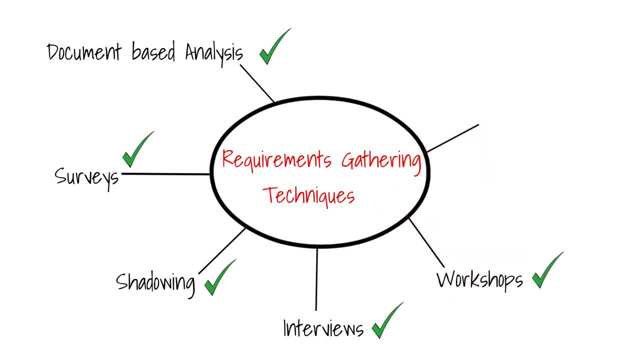 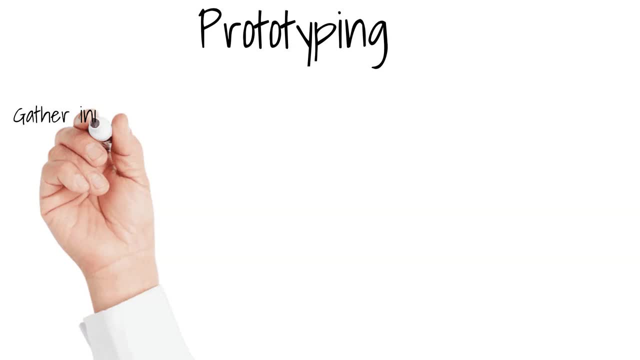 let me explain to you the last important requirements. gathering technique for business analysts: Prototyping. What prototyping is about is basically that you build an increment of your product or system based on the initial requirements, Show this increment to the stakeholder and, from there on, gather the next requirements. 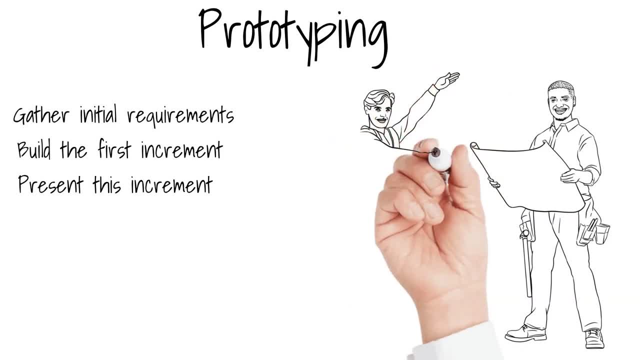 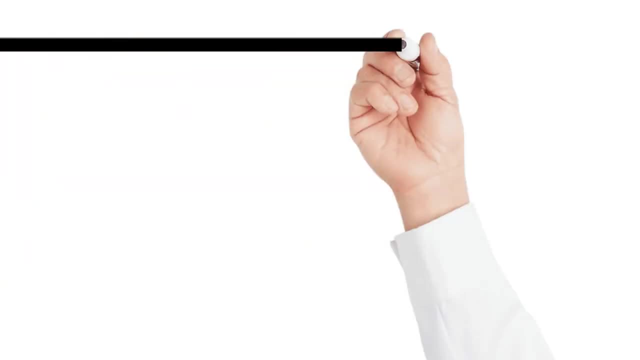 This is an iterative and incremental process. These concepts are part of the Agile methodology. Have you already worked with Agile and other methodologies? If so, let me know in the comment section below. After describing these requirements gathering techniques, I want to contrast them against each other. 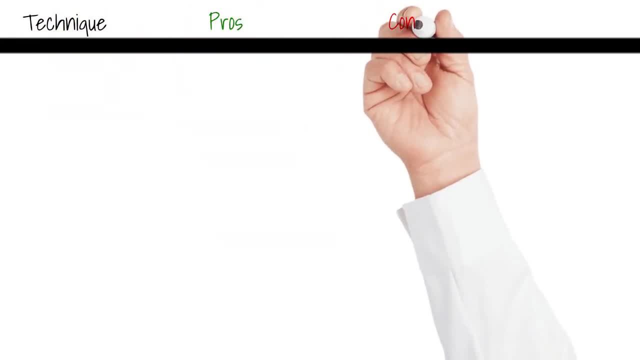 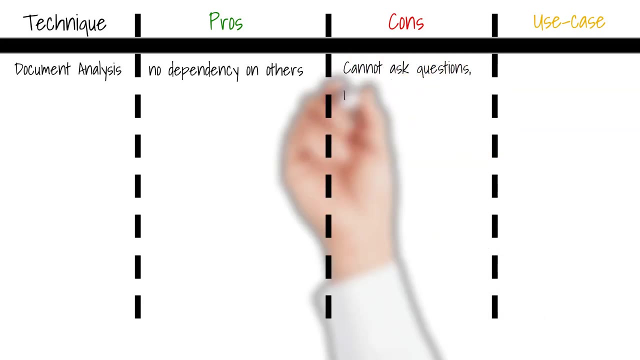 Let's talk about the pros, cons and use cases on when to use them and when not. Like I've mentioned in the beginning, document analysis has the pro that you are not dependent on others because the information is inside a document. The con here is that you cannot ask questions to this document. 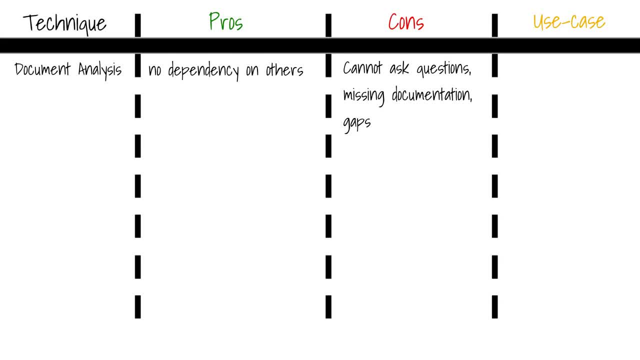 if there is something unclear to you or maybe any gaps. Also, in reality we often have missing documentation or even, like I said, gaps in these documents. The use case here is that document analysis is a good requirements gathering technique, especially for business analysts, for having a starting point or an entering point into the project. 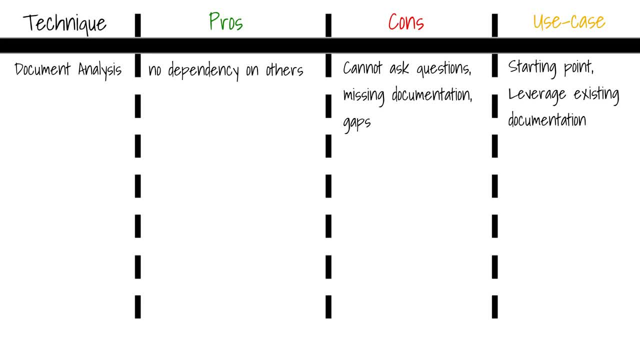 You can leverage existing documentation to build your baseline of know-how. That's good to get up to speed with the topic. Surveys, on the other hand, have the advantage of an easy evaluation of the data and also getting a lot of data. 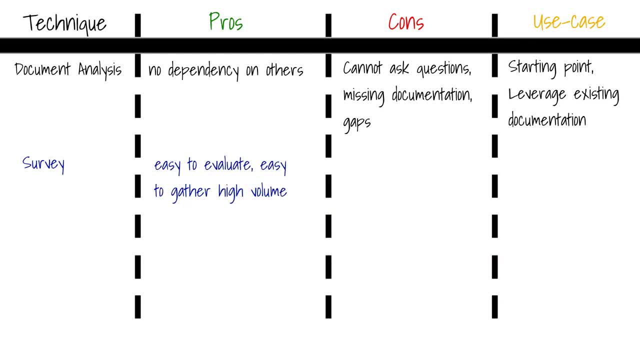 The issue, although, is we cannot get too specific in these surveys because people cannot ask questions to clarify something. The use case would be: if you want very generic information about the stakeholders or the use of a system or process, then surveys might be fine. 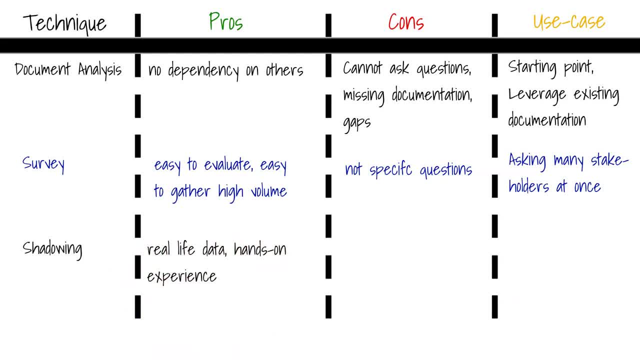 Shadowing has the huge advantage of gathering real-life data. You are able to get hands-on experience as you observe and shadow your stakeholder or future user. The con here is the time-consuming aspect for the business analyst. Nonetheless, this technique is useful when your stakeholder has no time for meetings with you. 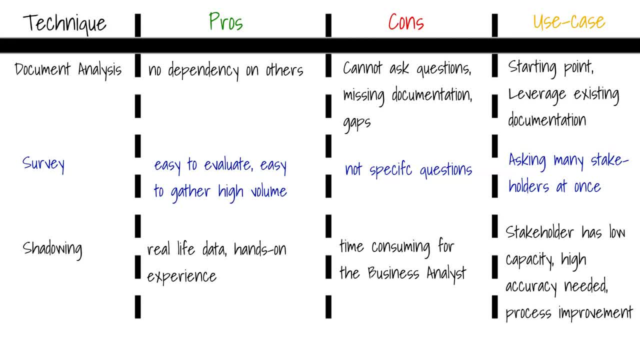 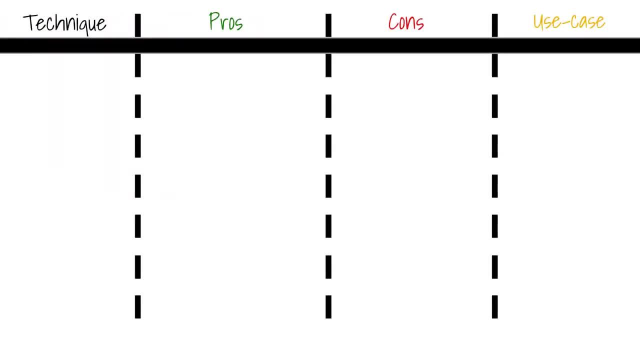 but it's fine to shadow him or her. You can also get a lot of data from the interviewer to get more insights. Especially for process improvement, shadowing is a very powerful technique. Interviews have the pro to get real-time answers and also to have follow-up questions. 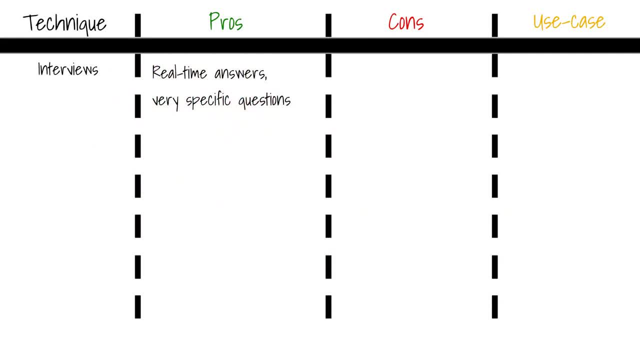 in order to get very specific. On the other hand, your stakeholder needs to have time for these meetings That also can get very time-consuming. Nonetheless, interviews are perfect to get more detailed requirements. Workshops have the pro that a big group of stakeholders is involved. 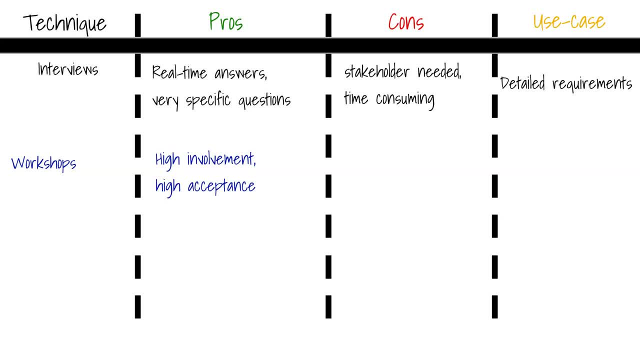 and the possibility to cover all the important requirements is higher. Furthermore, the acceptance from stakeholders is also higher because they are involved in the process. The con here is especially the time-consuming aspect. Full-day workshops with 10 people are very costly. In my experience, I used workshops in complex scenarios when we had inconsistent requirements. 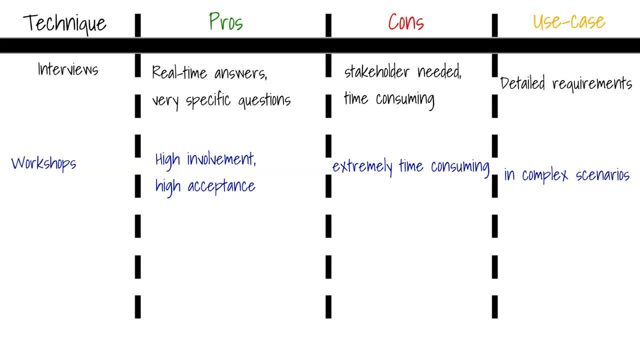 It helped a lot to bring stakeholders on the same page. Prototyping has the pro that you deliver something tangible with each increment. That helps the stakeholder to understand what we are doing, On the other hand, producing an increment each time and then going back to the stakeholder. 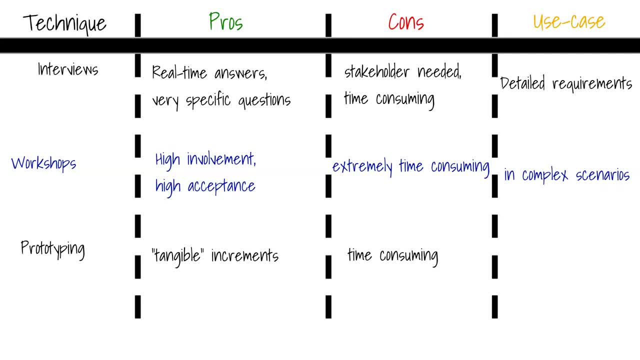 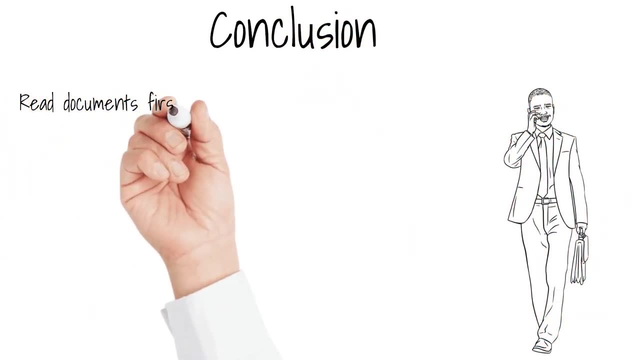 can get time-consuming. The use case is when you have unclear requirements but the stakeholder wants to see results frequently. Now let's summarize. Based on my personal experience, I would recommend to always start the document-based analysis. So read the documents to build your initial know-how.